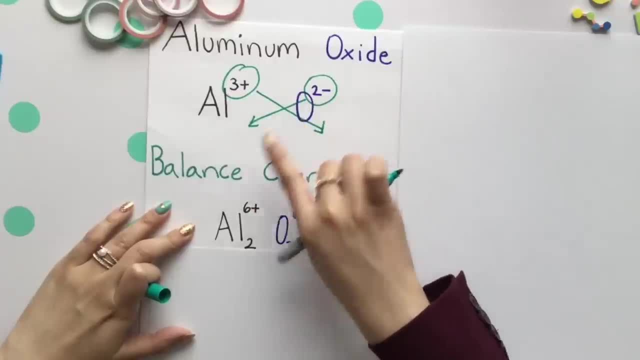 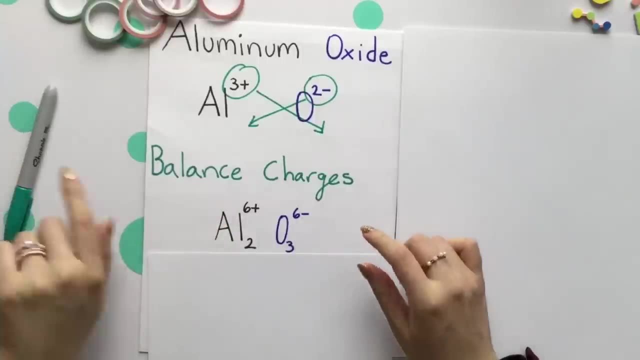 2 and oxygen then gets the 3. They get the opposite charges of each other, just so they can make the same amount of charge At the exact charge. they would then cancel out the charges and be neutral, and our final balanced compound is Aluminum oxide, having that subscript of 2 and 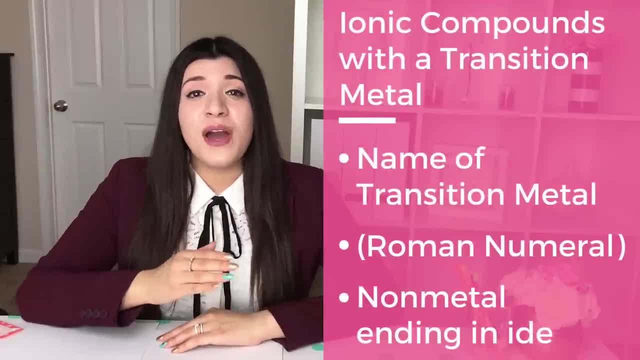 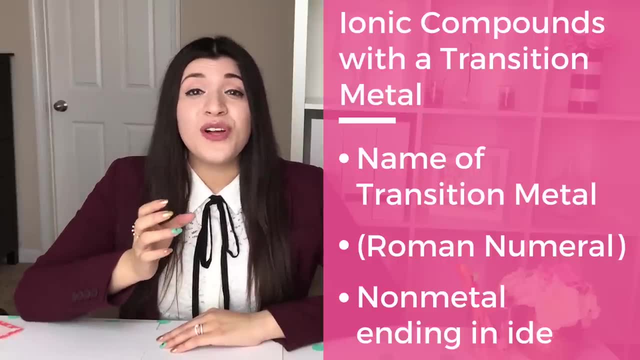 3.. The second one is Ionic compounds with a transition metal. This consists of the name of our transition metal, a roman numeral in parentheses and a non metal ending in Eid: our據谢谢 저희, Our. 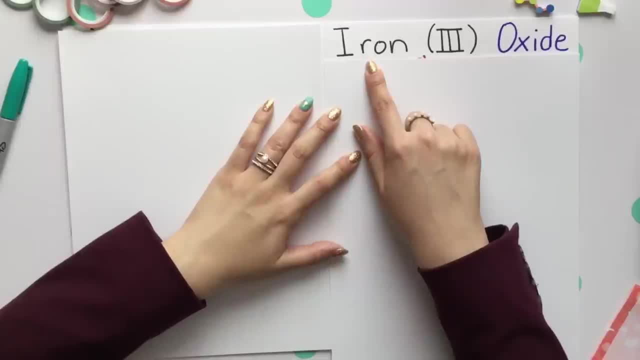 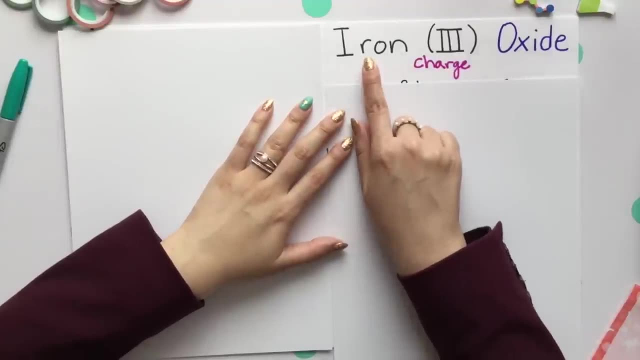 next comment: Outkit glaube. Our next comment품: transition metal is iron and our Roman numeral is three. Your Roman numeral actually tells you the charge of your transition metal. A lot of times transition metals have different types of charges. Iron sometimes has a two plus. 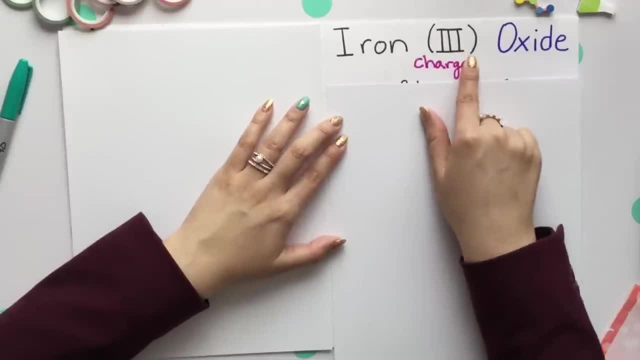 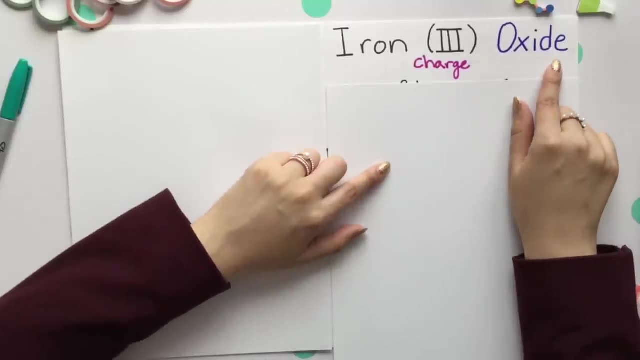 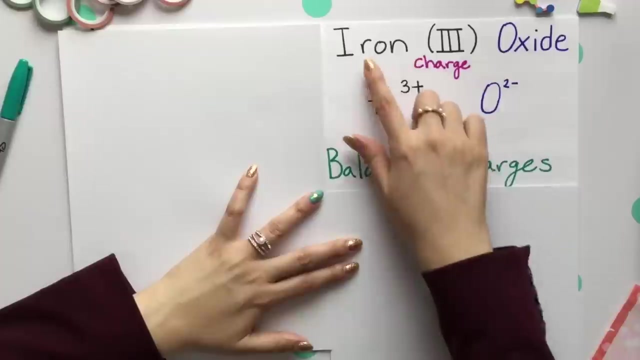 or a three plus charge. so our Roman numeral actually tells us the charge of what iron is within this compound. Your nonmetal is the oxygen and once again that ends in "-ide". So we need to balance out our charges. Your iron, as we saw, was 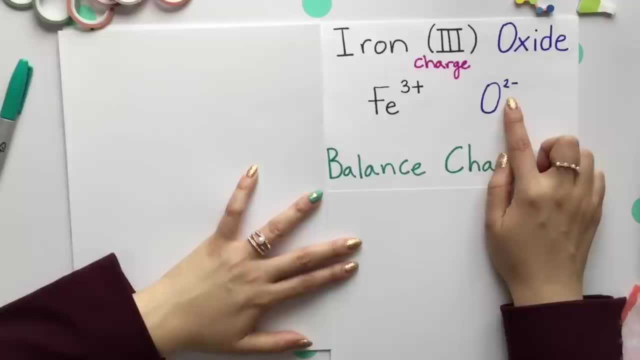 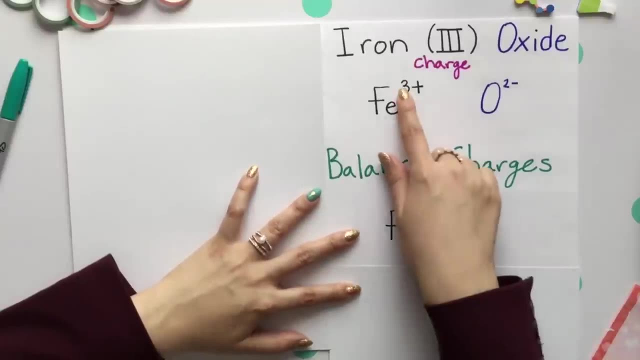 a three plus charge. Your oxygen was a two minus charge. Balancing out these charges will place a two subscript for our iron and a three subscript for the oxygen. We now have these sixes canceling out, which is what we wanted, and your final compound is Fe2O3. 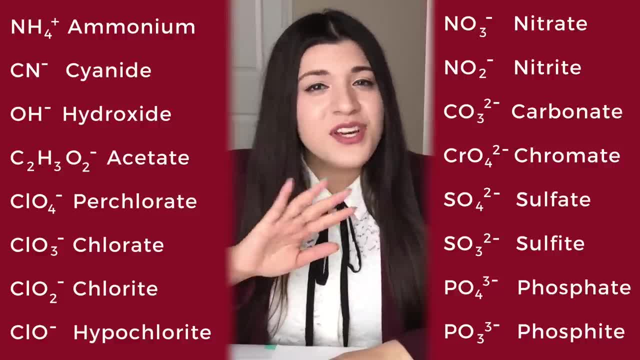 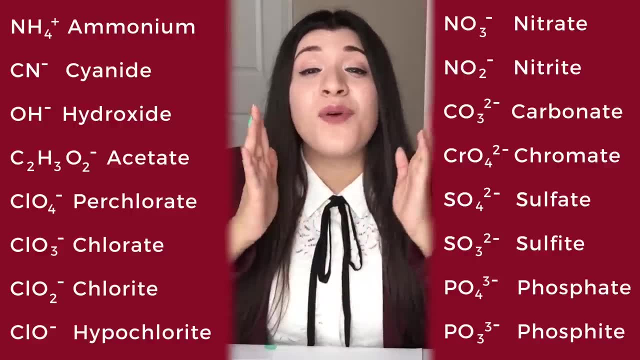 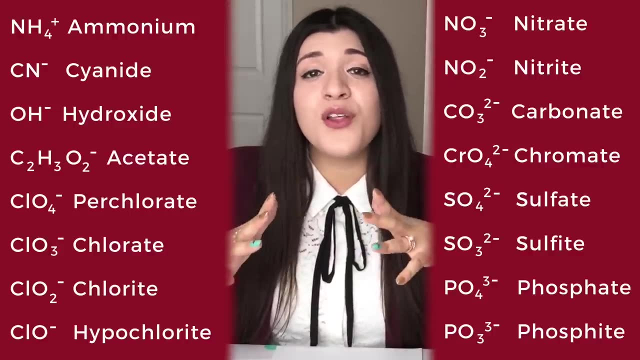 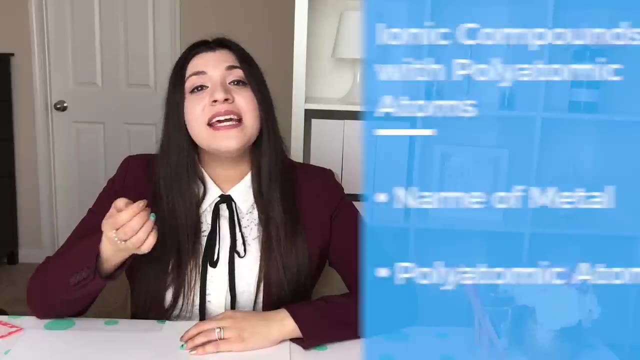 Polyatomic atoms just means that there are two or more elements within that atom. Know these polyatomic atoms, Write some flashcards. I will also place a link in the description box of more polyatomic atoms that you should also know. Moving on to ionic compounds with a polyatomic atom, They consist of the name: 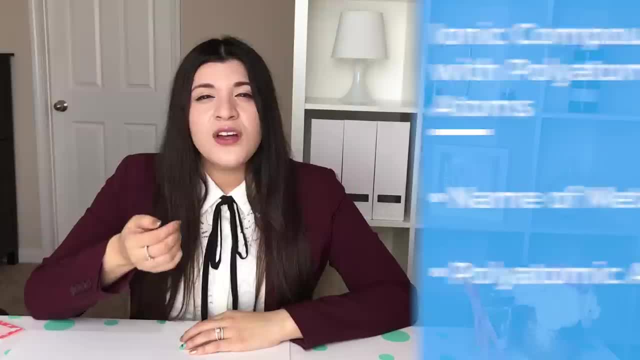 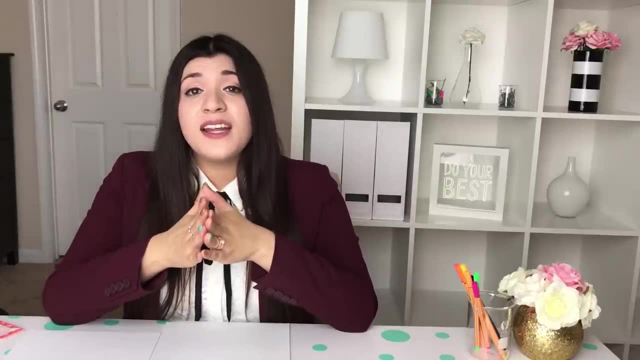 of our metal and our polyatomic atom. Notice that the name of our metal is not the same as the name of our atom. Notice that you do not have your nonmetal ending in "-ide". A lot of times polyatomic atoms end in "-ate or "-ite" With the 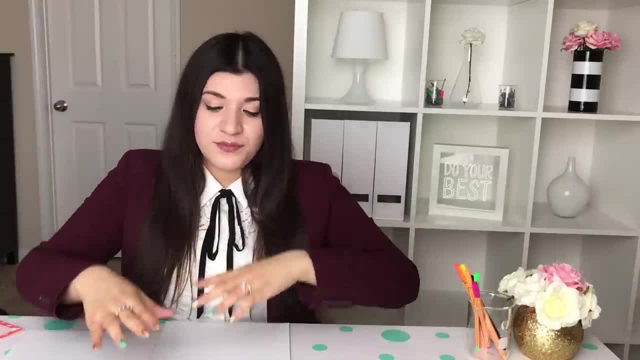 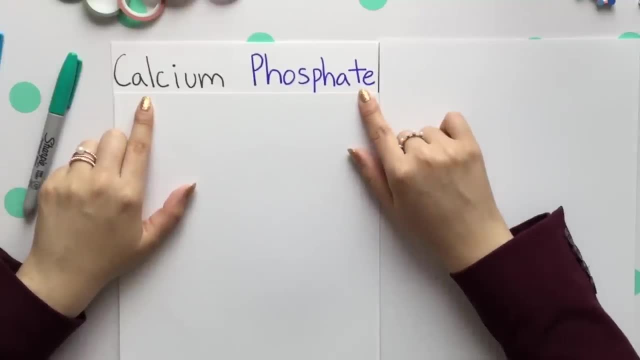 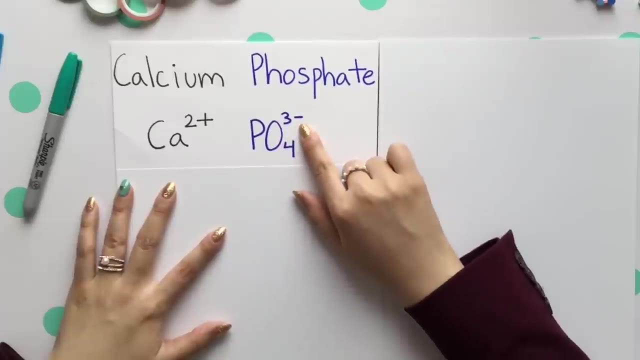 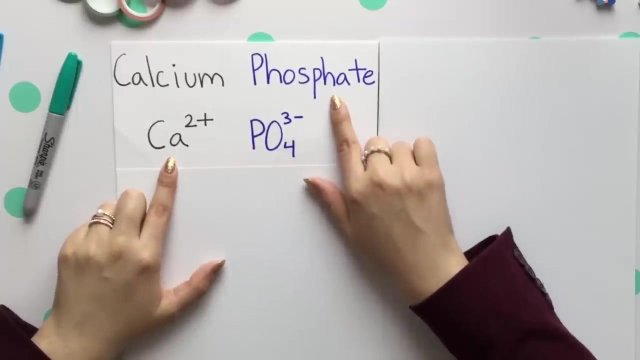 exception of hydroxide and cyanide. We have calcium- phosphate- Calcium is the name of our metal and phosphate is our type of polyatomic atom. Polyatomic atoms do have specific charges, so that is, once again, something you do have to know. Calcium has a 2 plus charge, Phosphate has a 3 minus charge. Our 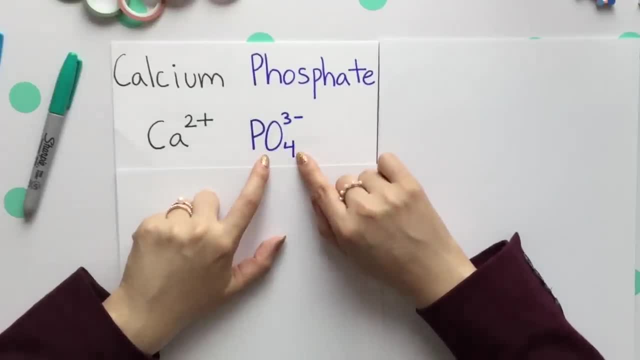 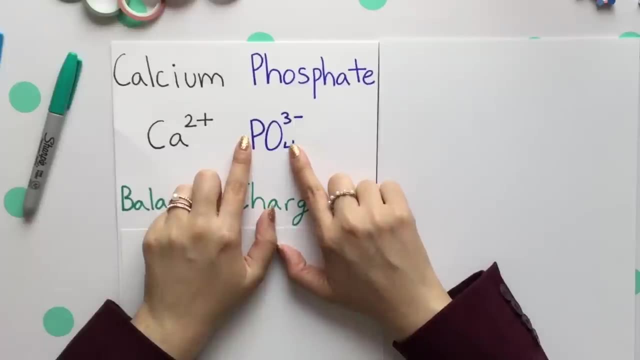 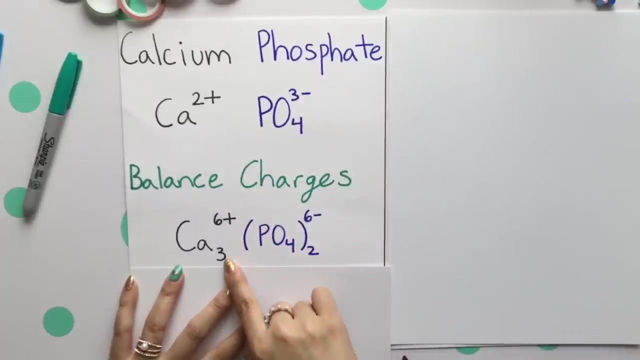 phosphate started off with having 4 oxygen. So to balance out our charges, we need to place this in parentheses to isolate that phosphate group. Doing so, we will place our 3 with our calcium. That will once again give us a 6 plus charge. 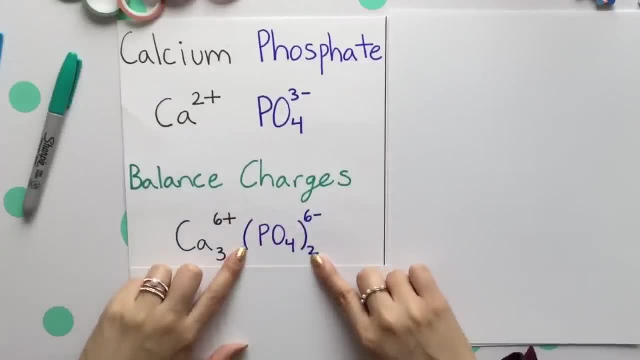 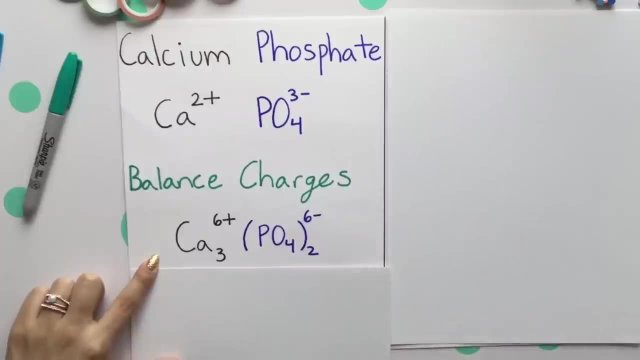 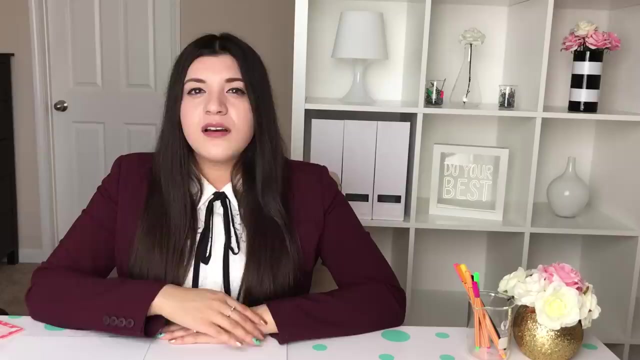 We'll place our 2 on the outside of parentheses. Polyatomic atoms tend to have parentheses whenever we place a subscript. These are now balanced And your final compound is calcium phosphate. This is how it's properly balanced. Our last ionic compound mixes transition metals and polyatomic atoms. 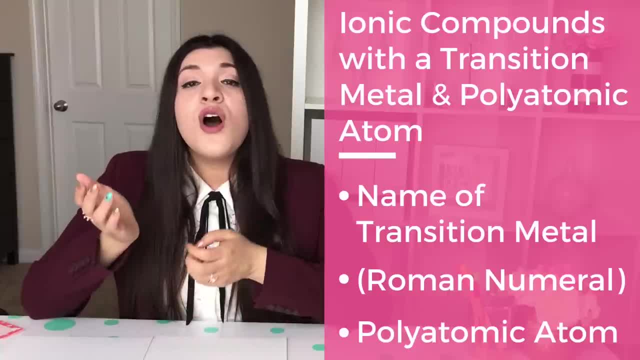 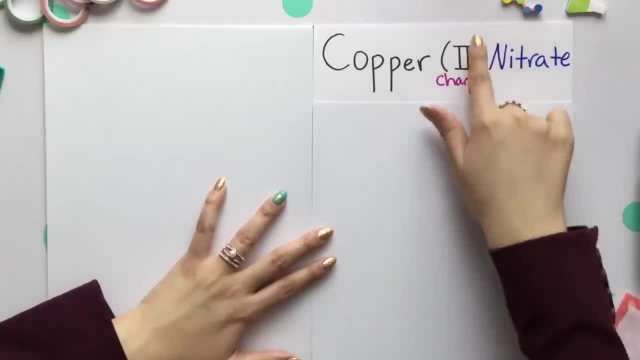 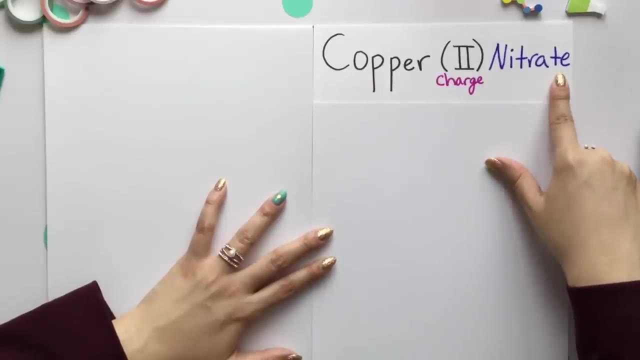 It consists of the name of the transition metal, a Roman numeral, and the polyatomic atom. Here we'll see copper 2.. Once again, that 2 tells us the charge of copper, which is our transition metal, and our polyatomic atom of nitrate. 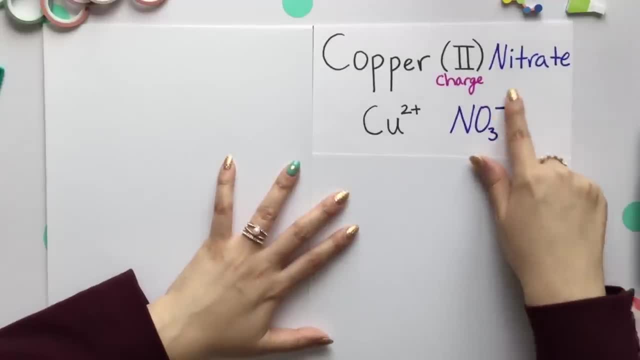 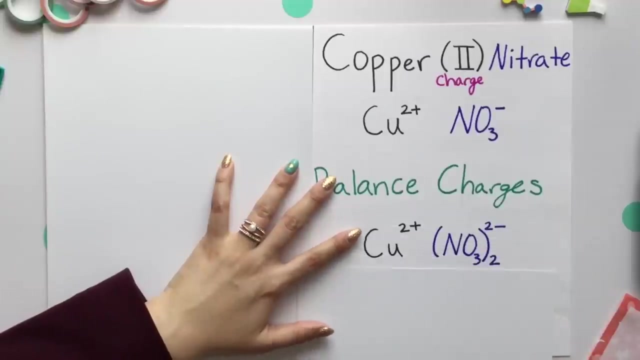 Nitrate is NO3 and has a negative 1 charge. We saw that copper had that 2 plus charge, so all we need to do is just have a 2 for our nitrate, since copper is already 2.. Balancing out our charges. 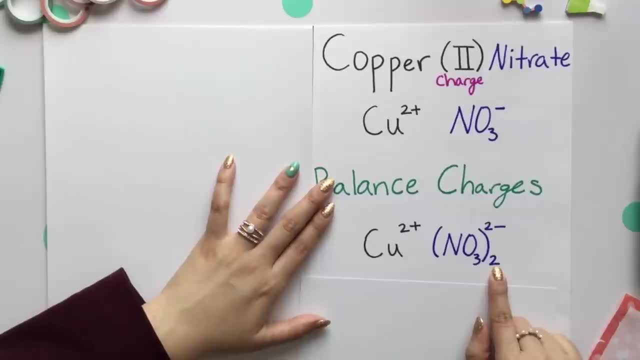 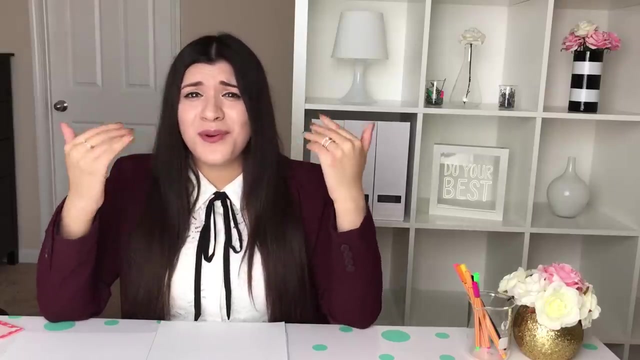 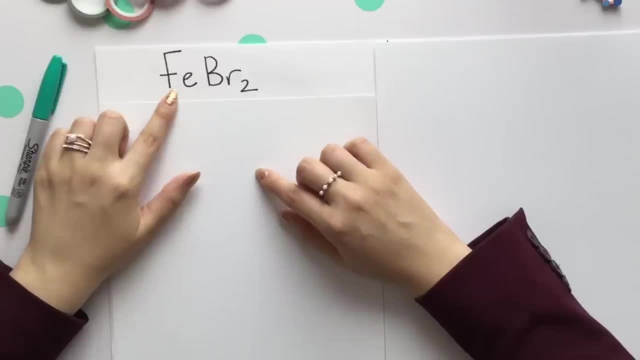 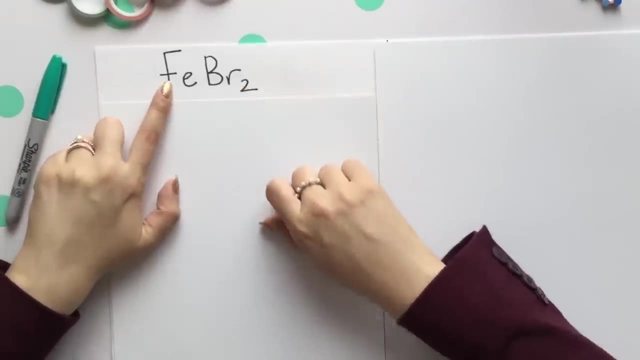 we're given the name of the compound name and asked to actually write the name of the compound, FeBr2.. Fe is known as iron and Br is known as bromine. Iron is a type of transition metal. Bromine is a nonmetal. 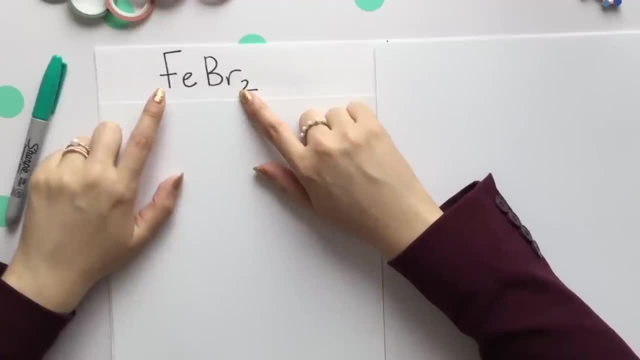 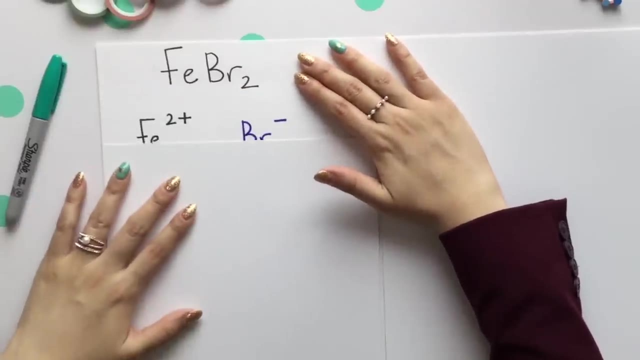 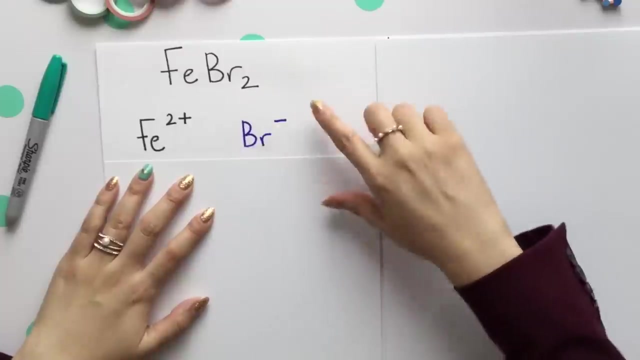 So our nonmetal will end in "-ide" and we know that a transition metal will have a Roman numeral. To figure out what your Roman numeral is, let's go back to the overall charges. So bromine is a type of halogen, just meaning that it has. 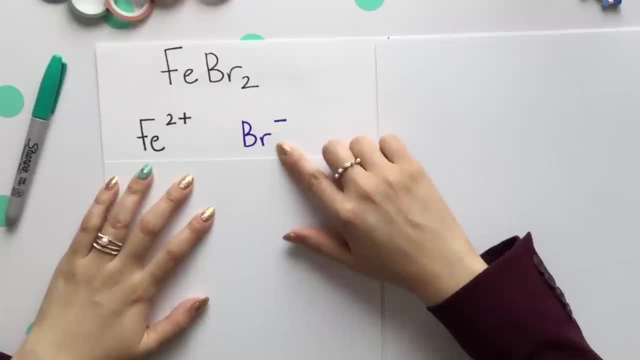 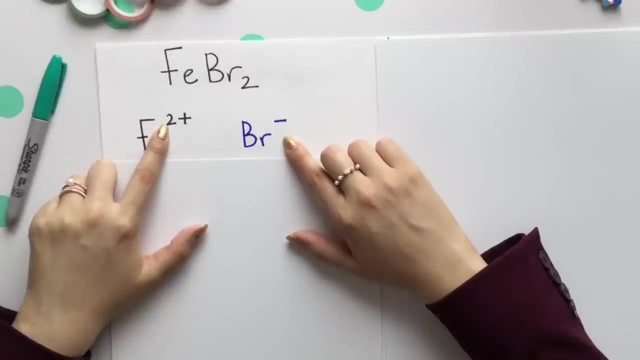 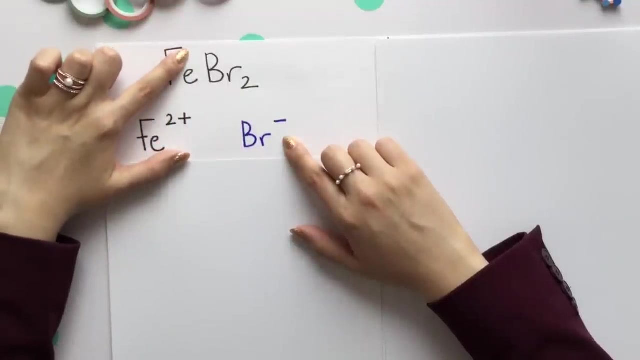 a negative one charge. So since this had a negative one charge, Fe or iron must have had a two plus charge. Another way of identifying this is, if we were to go backwards, this two would go back onto the iron, since bromine needed two to balance out the charges altogether. 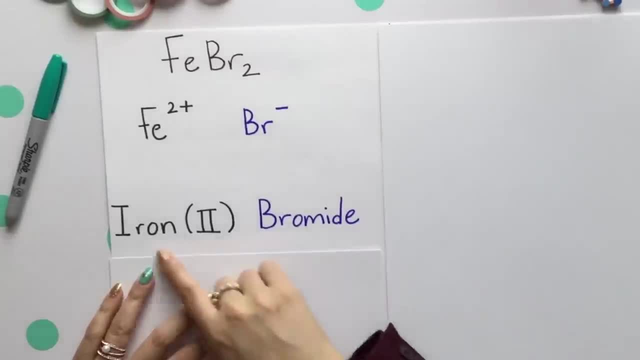 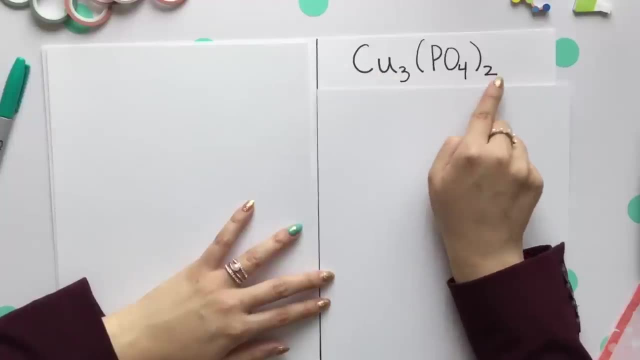 So we'll have iron to bromide. Let's try another example like that: Cu3PO42.. Cu is known as copper. It is a type of transition metal, So we have to have a Roman numeral. PO4 is a type of polyatomic. 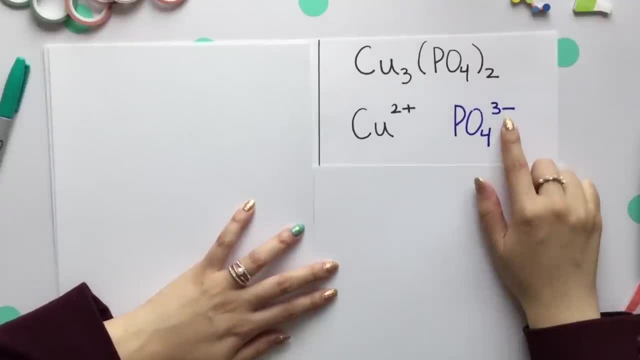 atom. We had to know that polyatomic atoms charge was a three minus because of the negative one charge, So we'll have iron to bromide. Let's try another example like that: Cu3PO42.. Cu is known as copper. It is a type of transition metal, So we have to have a Roman numeral. 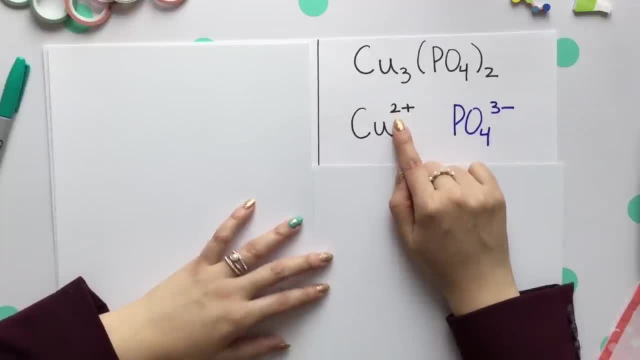 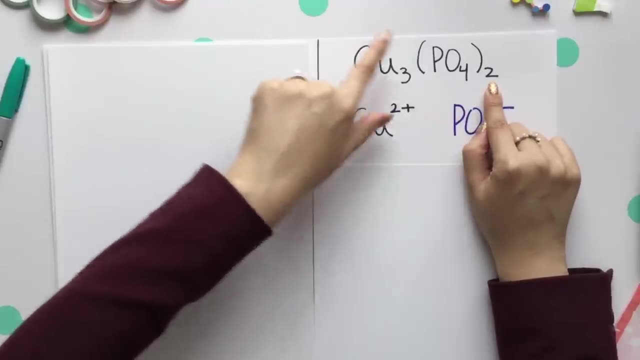 Because this then allows us to figure out that copper had a two plus charge. Another way of looking at this is this: two goes back to the previous element, So that two belongs to the copper and this three then belongs to our phosphate group. That's a trick that you can use whenever. 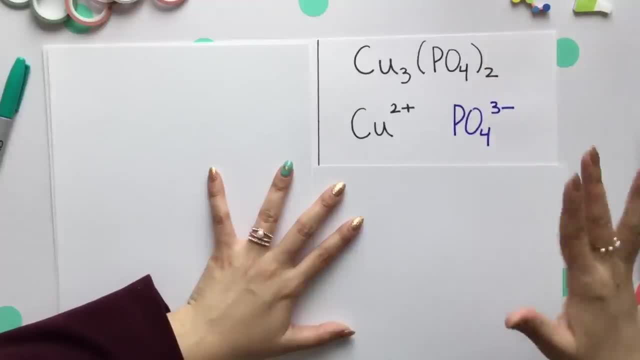 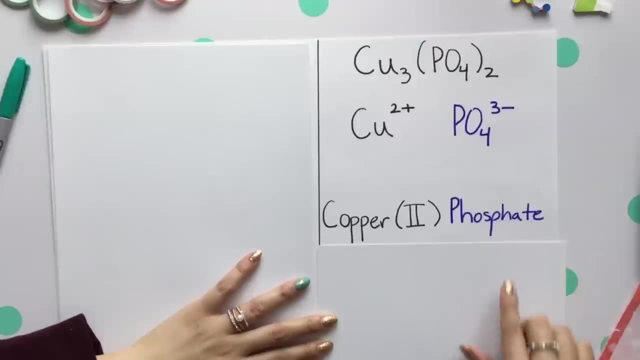 you're using your formula and you're trying to go back to the actual name of the compound. So our name of our compound would then be copper 2-phosphate. Those are all the different types of combinations that we can use. So let's try another example: Cu3PO42.. Cu is known as copper. 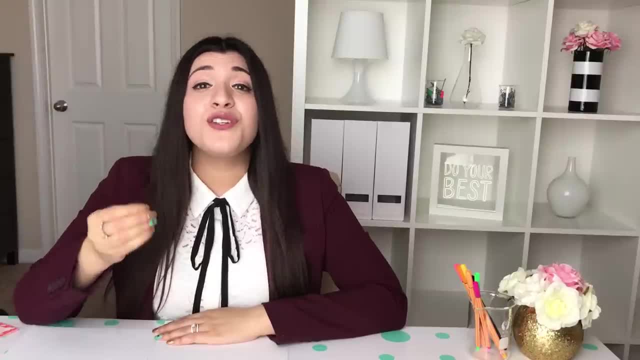 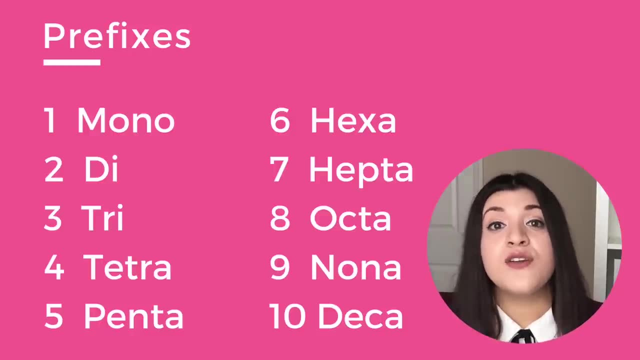 U3PO42.. Cu is known as copper. It is a type of transition metalhopping Moving on to covalent or molecular compounds. Something that we have to know are the prefixes. Know one through ten, because you do not have to balance any of the charges. I repeat, for covalent.